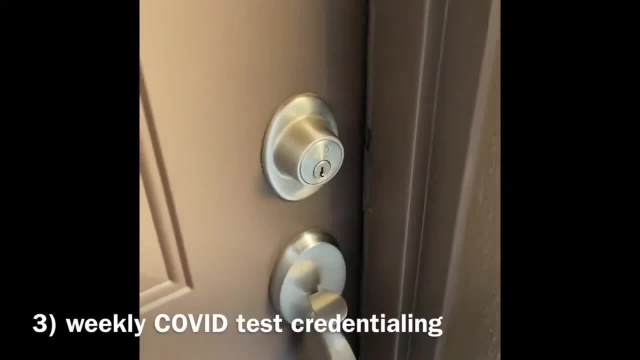 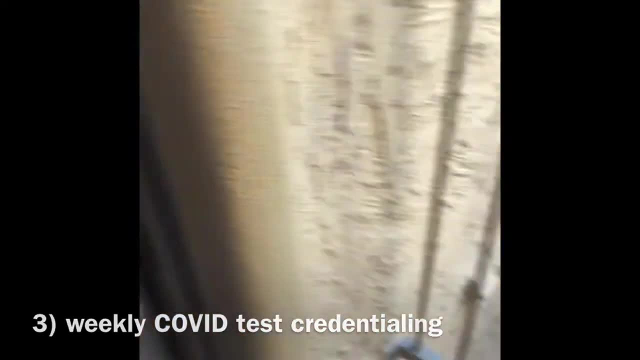 about it the morning of Third thing I'm thinking about: I need to get COVID tested tomorrow morning as part of weekly credentialing for one of the surgery centers I support. And then another thing I'm thinking about is being on New Year's Eve call, So again stocking up on product, making sure I'm calling. 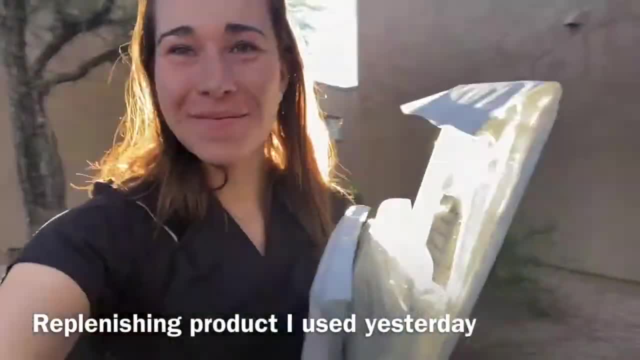 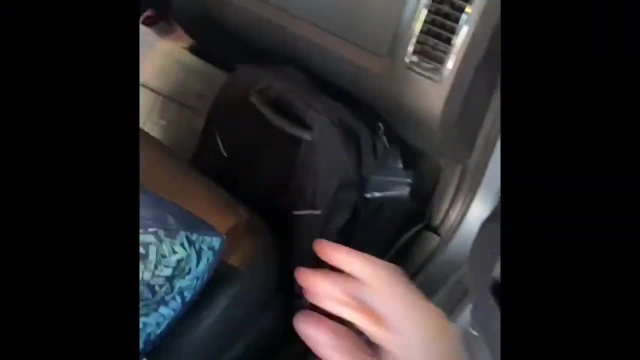 ahead. We are only allowed to do ground shipping right now, which takes about four days. So lots of planning going on, But most importantly, I'm thinking if I have enough gas to get to my first check out West. Let's see. 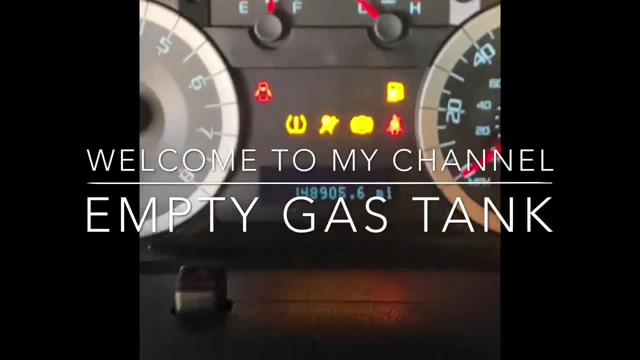 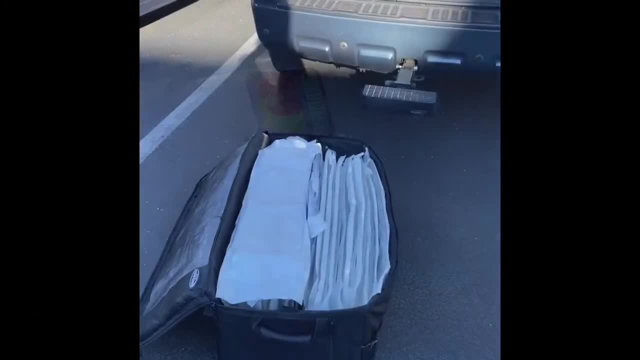 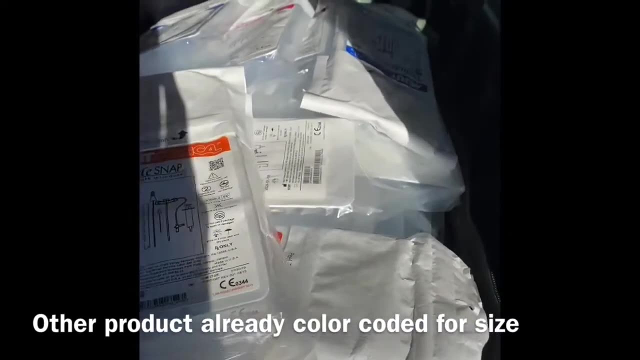 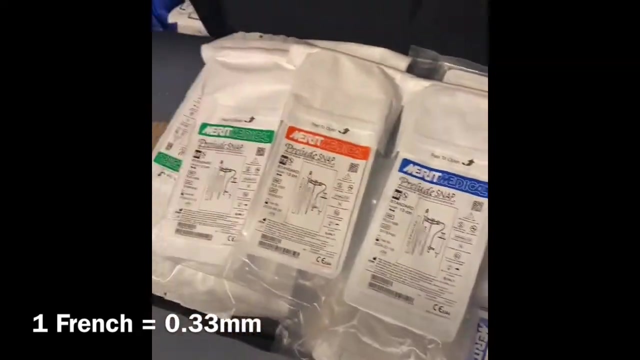 Sometimes it's hard to differentiate the product when it all looks the same. A trick I use is stickers, So there's two systems in here, but stickers help me make sure I don't drop the wrong size. Talking about size, these are sheets. They are measured in French size One French is. 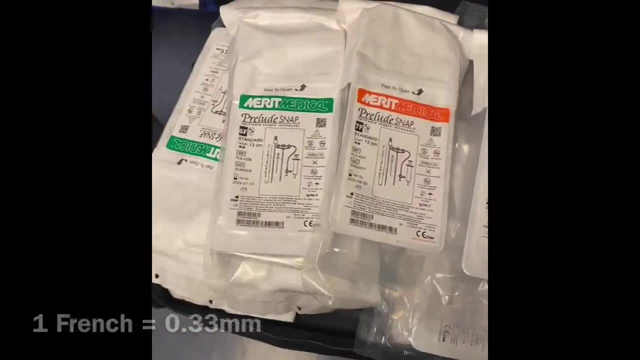 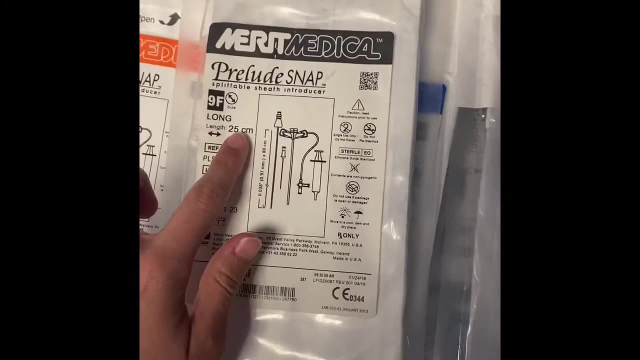 equivalent to 0.33 millimeters. So I'm going to take one of these and I'm going to take one of these, so I don't need stickers for these, because they're color coded. And notice, we have two different lengths. We have a long which is 25 centimeters and then our standard 13.. Okay, so let me show you. 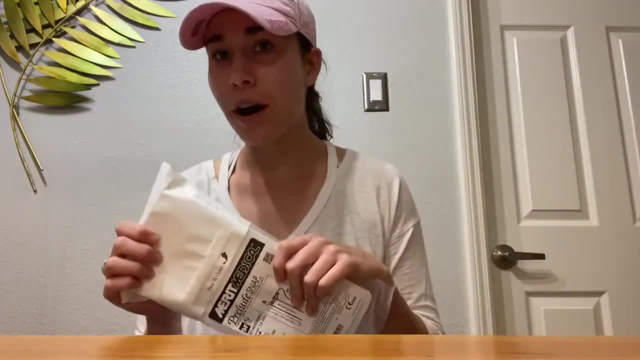 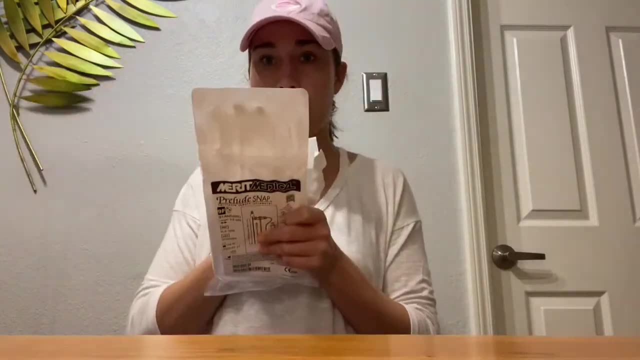 what a sheath is. So obviously I'm not in scrubs, but you'll open this in sterile fashion. So what that means is opening away from you, And you can either hand that off to the scrub tech or imagine this is the scrub table. 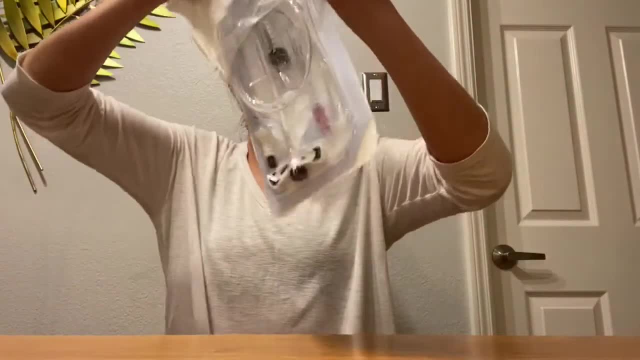 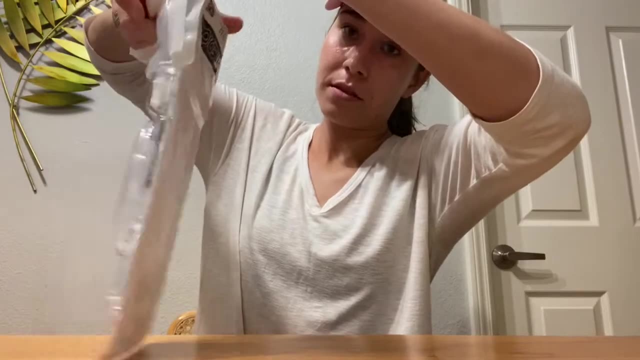 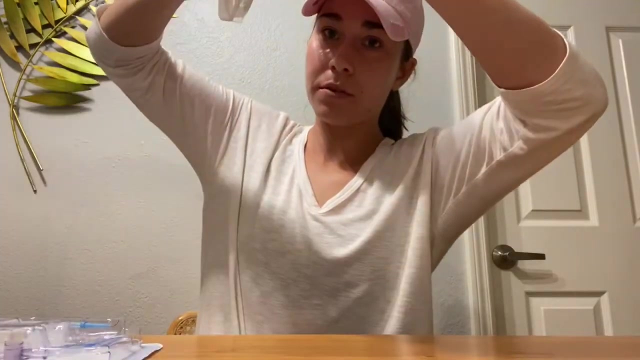 I'll inch it out. as far as I can Notice I'm not touching anything, And then I'll give it a tip. So imagine this is sterile. It would be blue. I can wiggle this onto the scrub tech's table. You want to give it a ledge and then it. 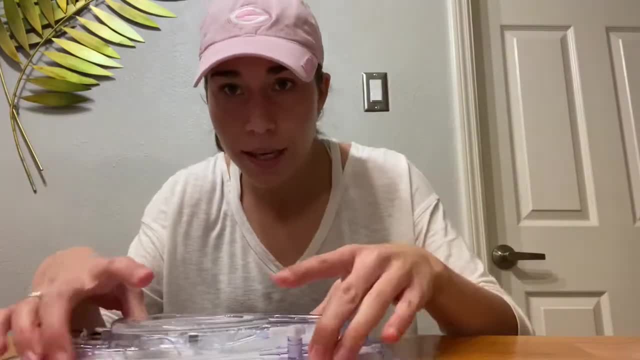 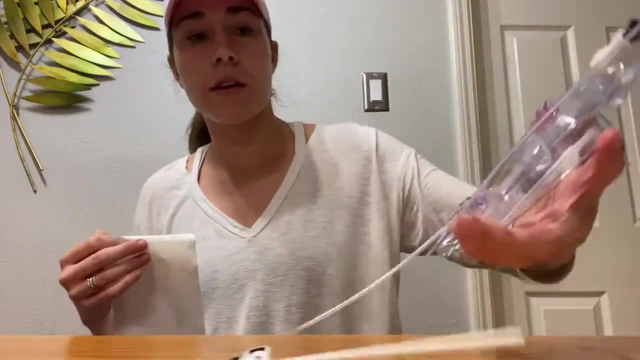 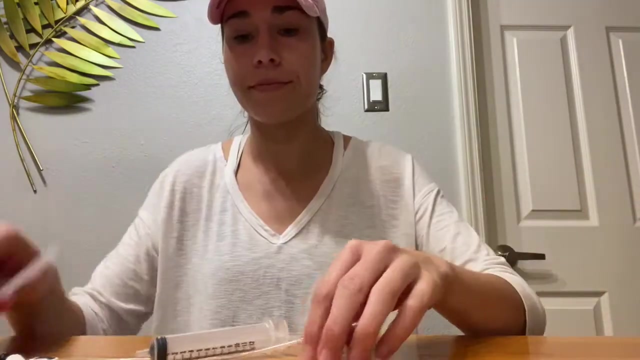 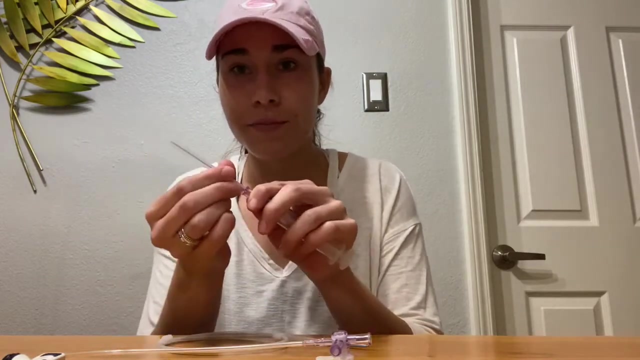 falls down flat so it doesn't go anywhere. And then the scrub tech's going to take the sterile sheet, open it And then still something in it. This is the wire. So if I'm prepping to implant a pacemaker, I'm going to put on this needle and then I'm going to fill this up with some, with some saline. 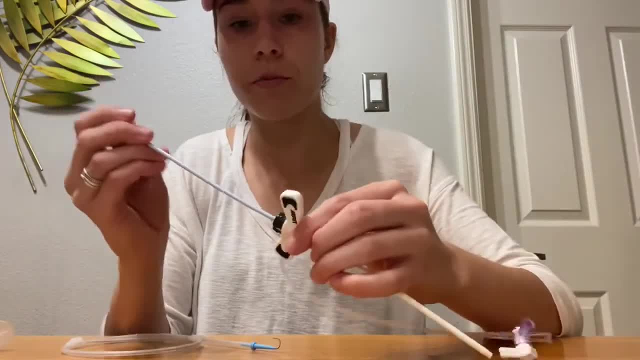 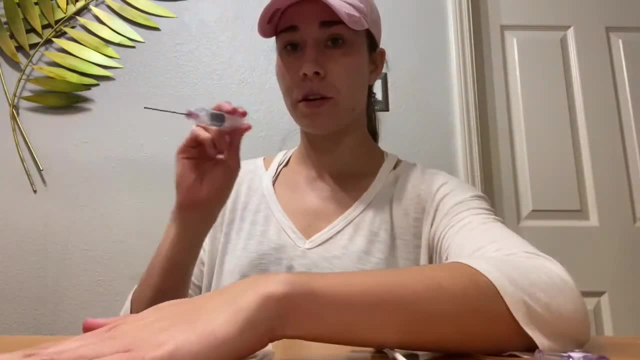 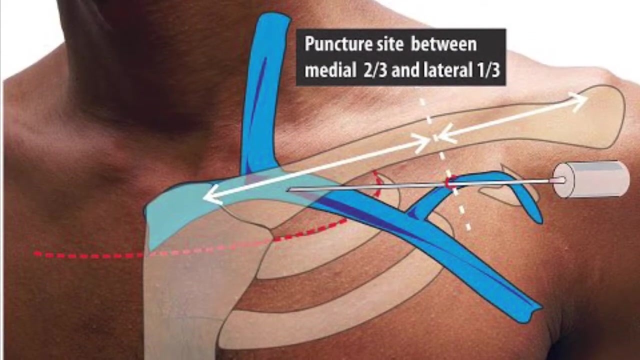 So prepping that with some saline- Sorry, prep my sheath That's going to be in there together. So this is the patient. We're using the needle, We're aiming at the cross section of the clavicle bone and the rib so that we don't puncture the lung. 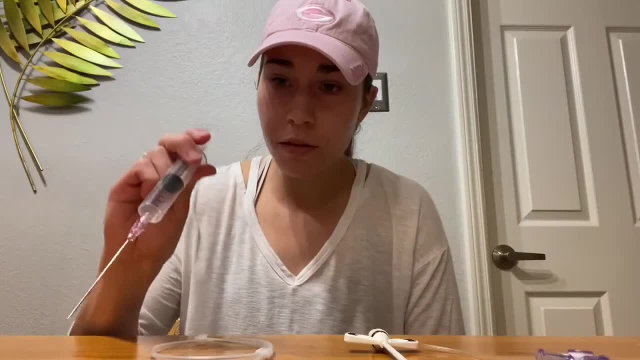 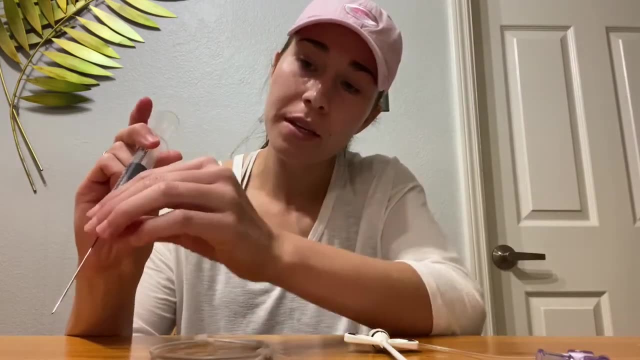 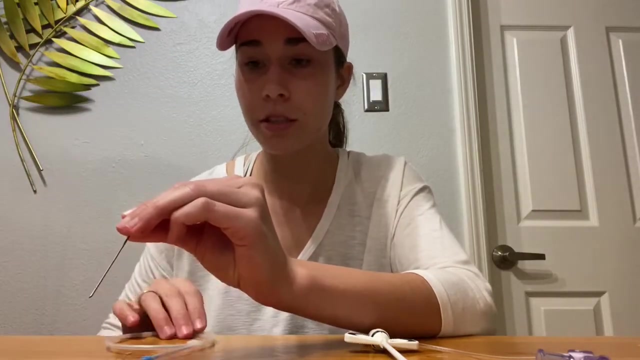 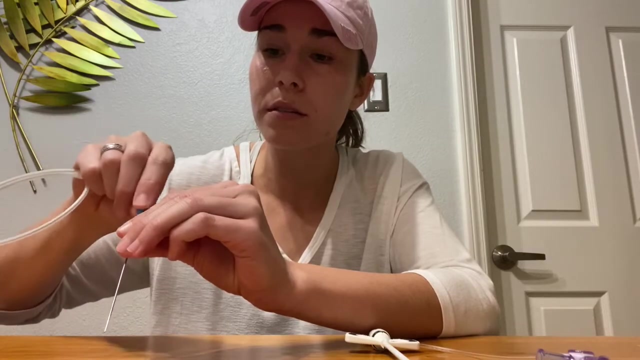 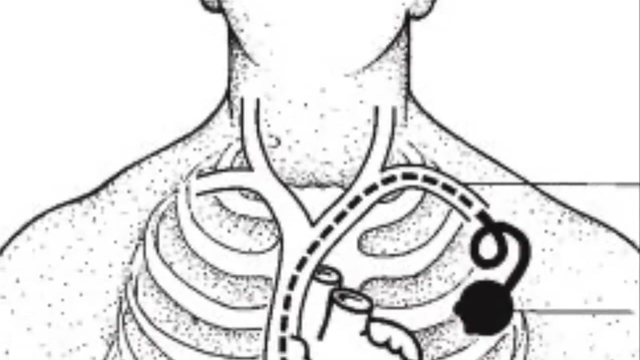 Kind of going to go at different angles until, boom, you're going to see a flash of red blood, venous blood. So what I'm going to do is I have access in the vein to take away the syringe. I'm going to take my wire, straighten it a little bit and I'm going to feed the wire into the vein. 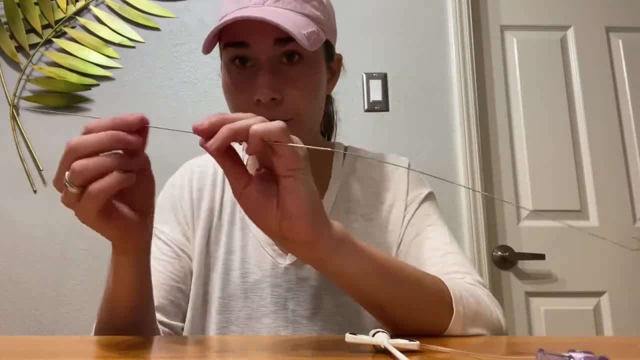 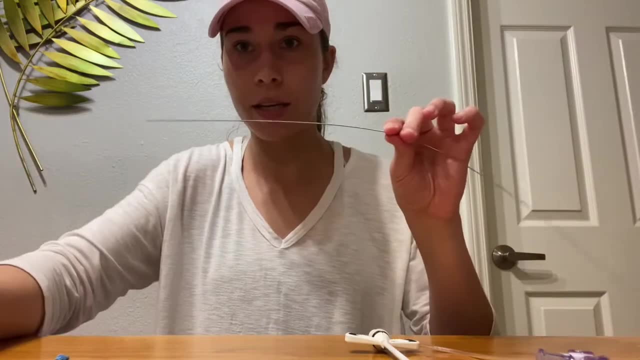 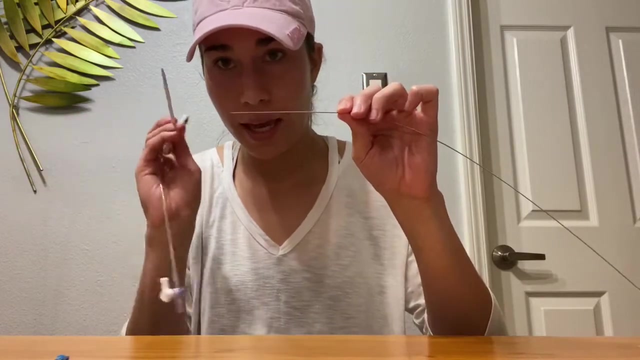 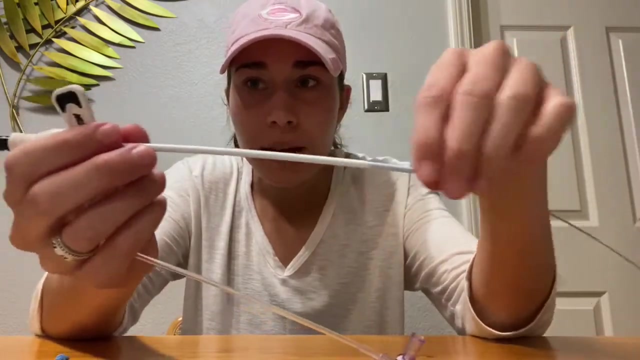 Okay. So now I have venous access, I can remove the needle. I'm retaining the wire. Now I'm going to aim my dilator and sheath. Okay, So this I'm in the vein. I got venous access. 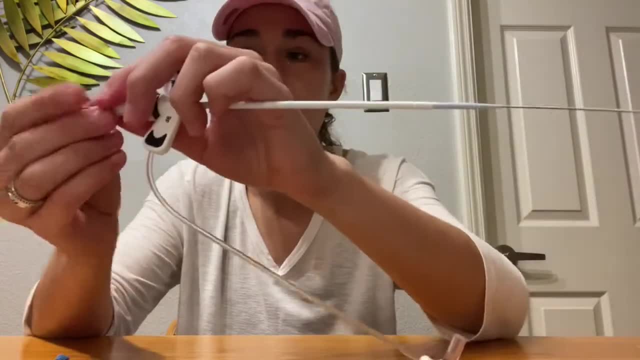 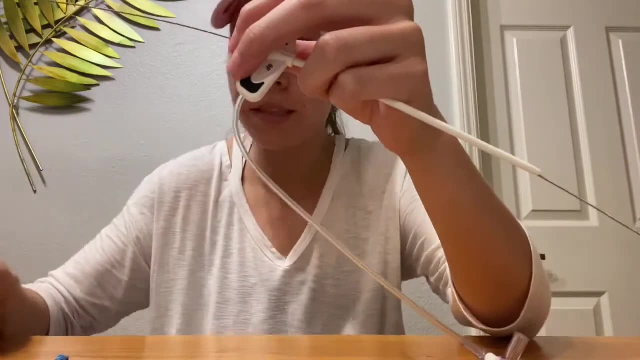 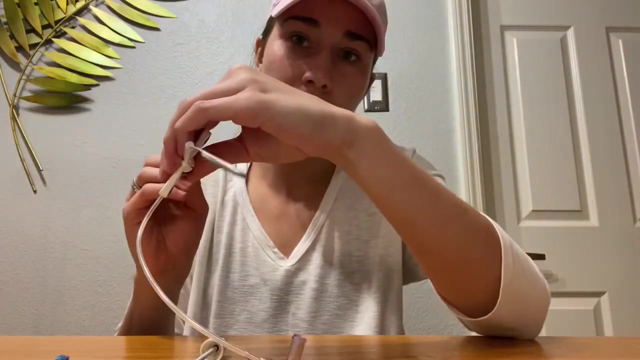 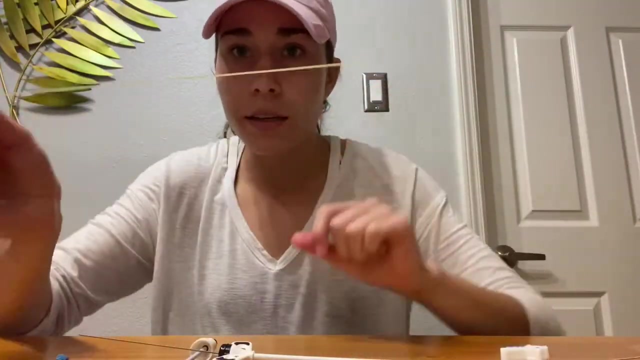 So I started off with the size of the needle. after I removed the dilator, See, it gets bigger and bigger, a little bigger. Now I'm nine French. So what's going to happen is I'm going to take my lead. I'm using a spaghetti noodle for this demonstration. 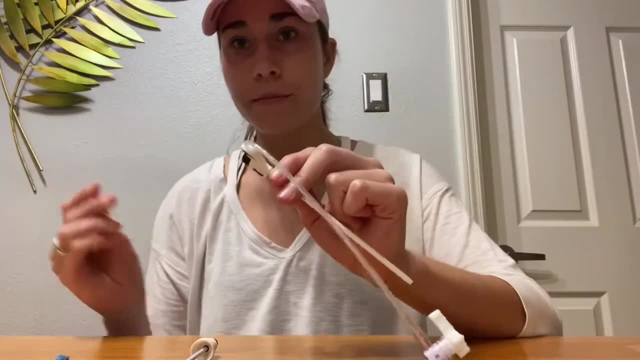 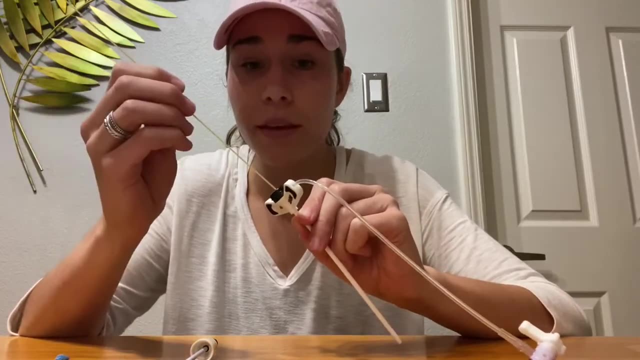 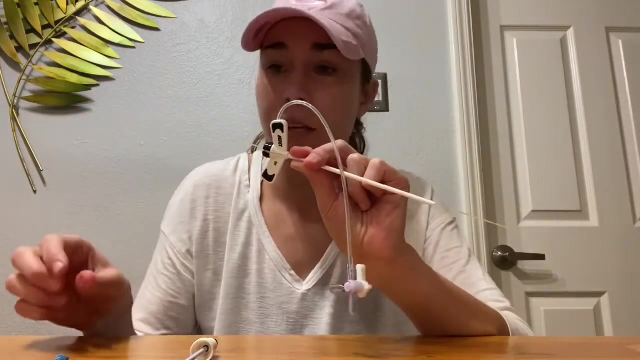 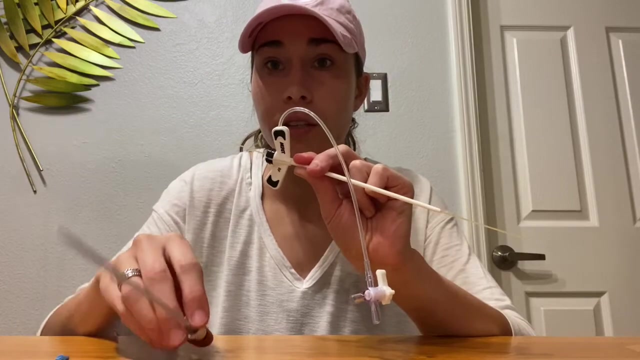 So now I don't need the wire anymore. I have nine French sheath access And if I have a nine French lead that'll fit in the sheet. So now I'm inserting the lead into the vein. So it took a needle, then a wire, sheath access. 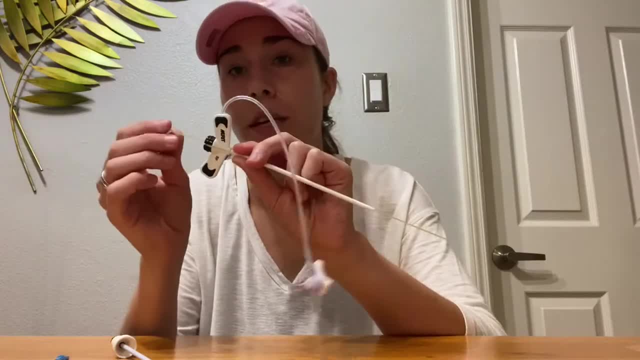 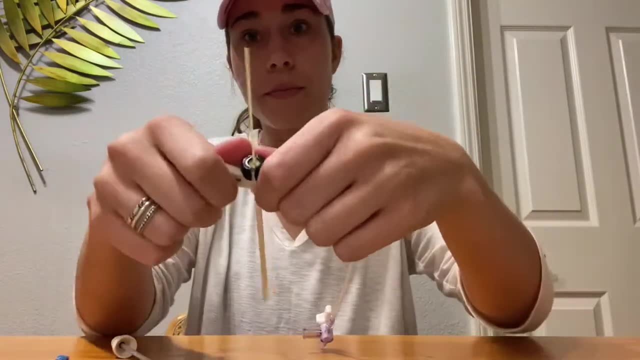 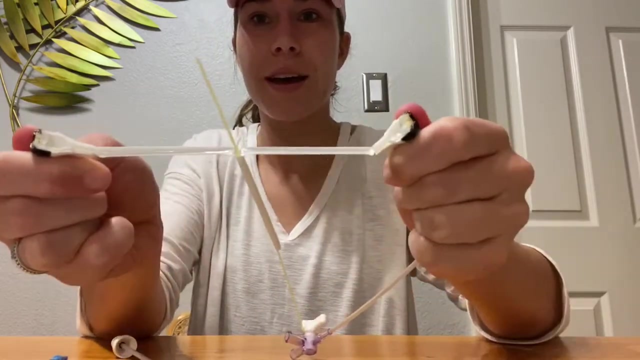 I have this sheath and I can feed my wire into the heart Once I place it. what do we do? We break this sheath. It's a peel-away. It has little butterfly wings. I'm just going to snap, peel it away. 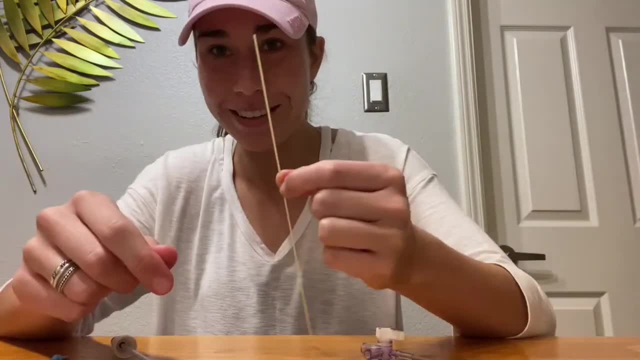 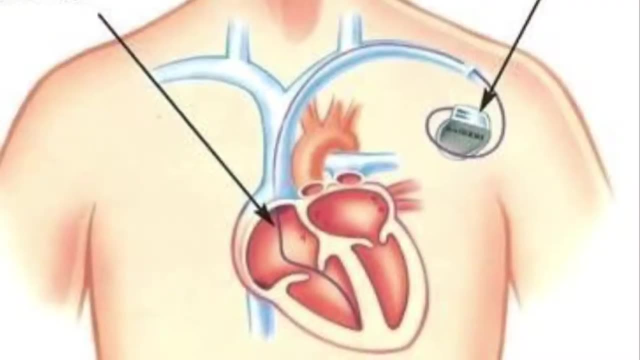 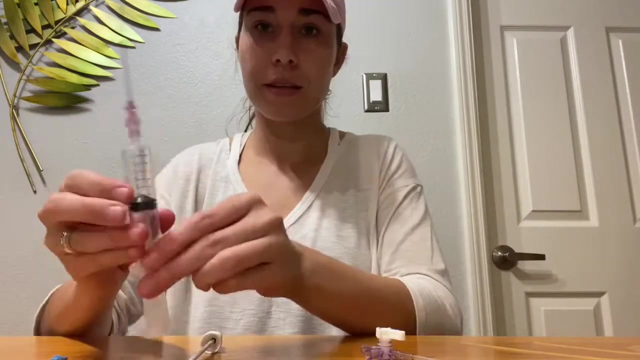 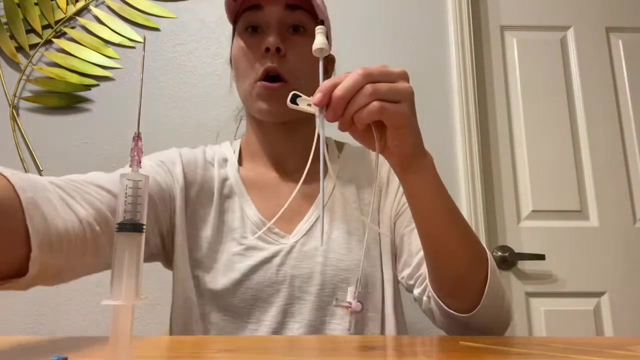 Boom And the spaghetti noodle would be retained in the venous system in the heart. That is how we fit a wire into our tiny venous system. So we do all that with accessing the vein using the sheath and dilator over a retained wire. 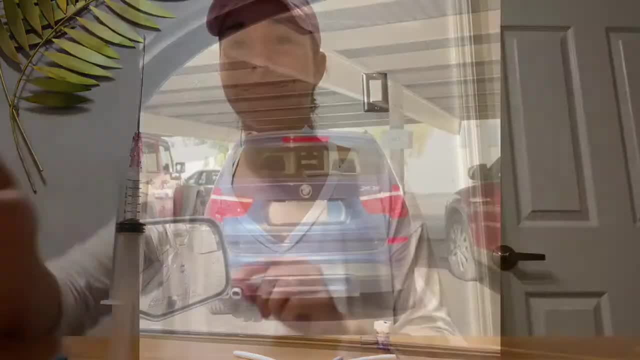 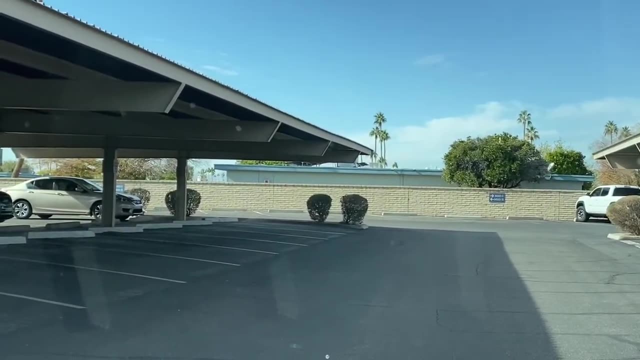 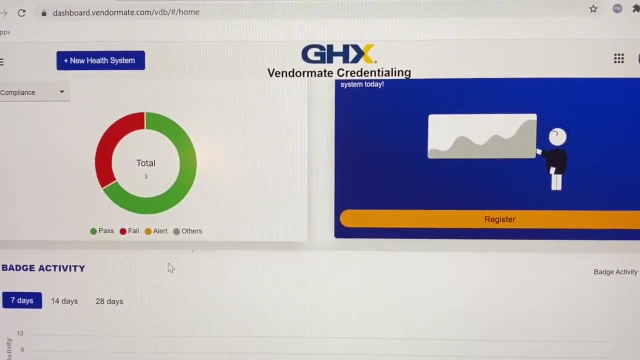 All to insert my lead. I look forward to explaining to you all how, at this one clinic I often go to, my car was keyed And there was nothing the police could do about it. unfortunately, Hospital credentialing has never been as important until this year, during the pandemic. 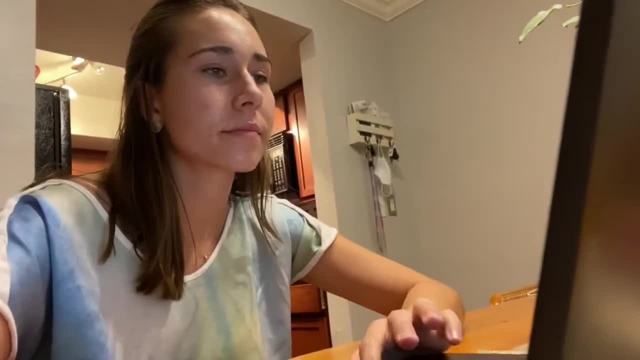 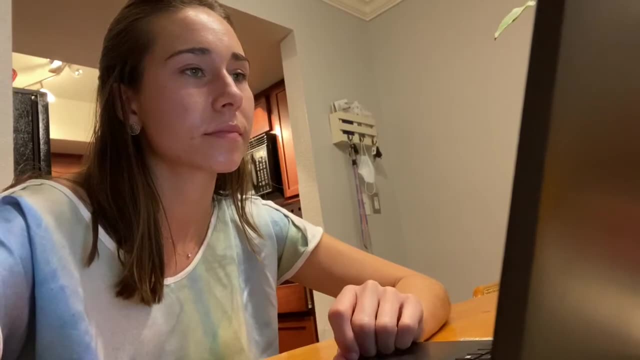 This is a way for hospitals to safeguard who is entering their hospital. I have four different credentialing accounts that I keep up to date with. This was an example of vendor meet. It seemed as though each month there's a new policy to sign or a credential that was nearing expiration. 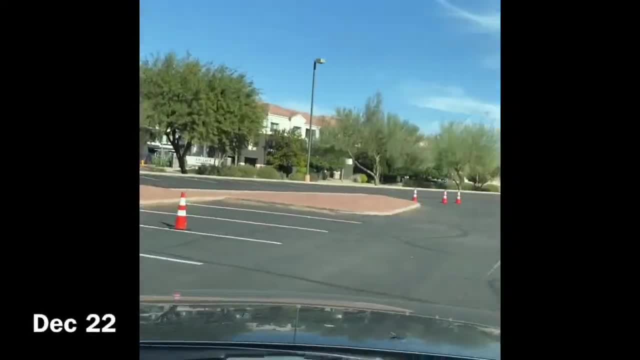 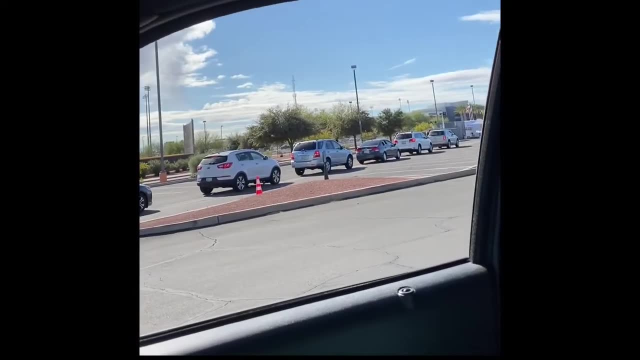 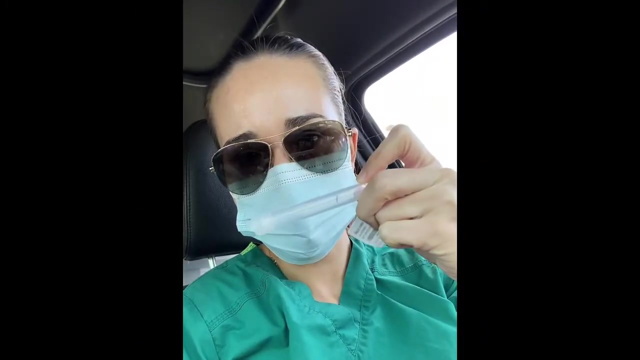 Tuesday after clinic I went to a nearby COVID testing site to get my weekly COVID test. One of the surgery centers requires a weekly negative test result to enter their facility. I just want to give a shout out to all the workers that make this possible. 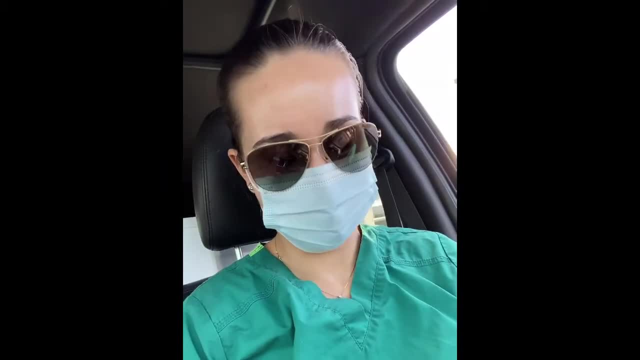 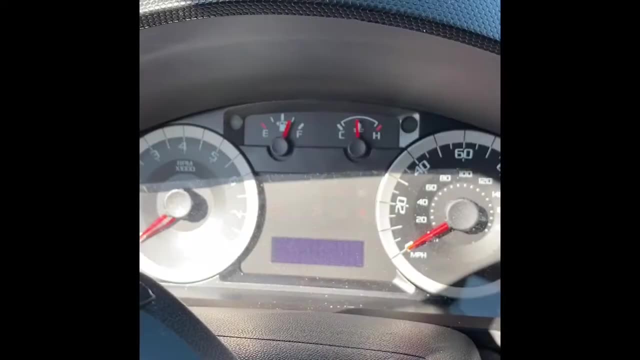 It's such a smooth process. I make an appointment beforehand, Roll up, They give me a test tube. They started doing saliva tests, So this tiny tube I have learned to perfect spitting into. Once you're done, you turn on your hazards. 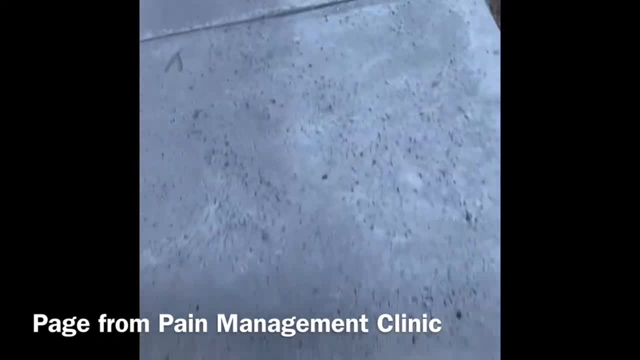 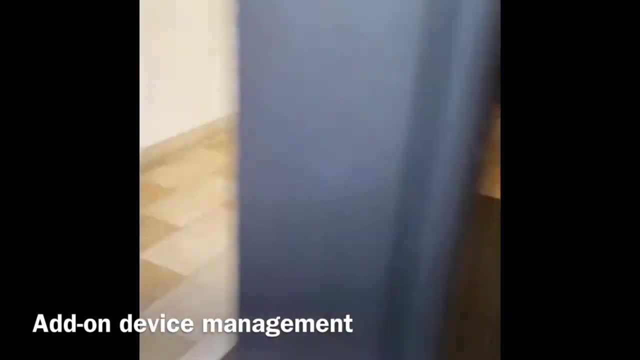 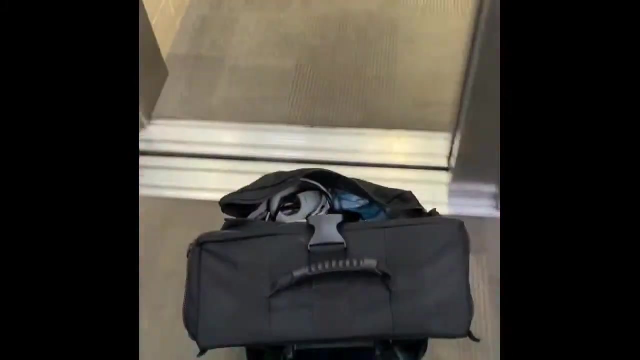 Someone comes and picks up the tube and you're all done. Device managements: These aren't as glamorous. As a biomedical engineer in the clinical field, I am looked to for pacemaker management as well as defibrillator management. One of our patients is having a heart attack. 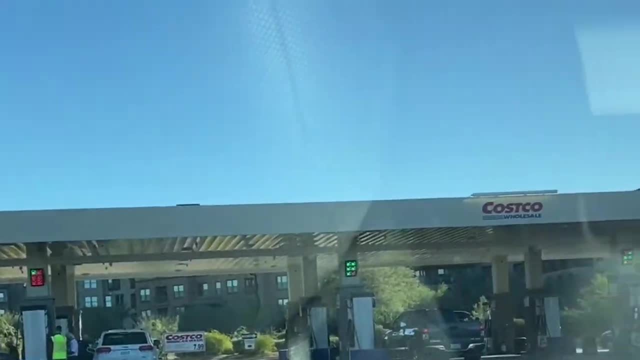 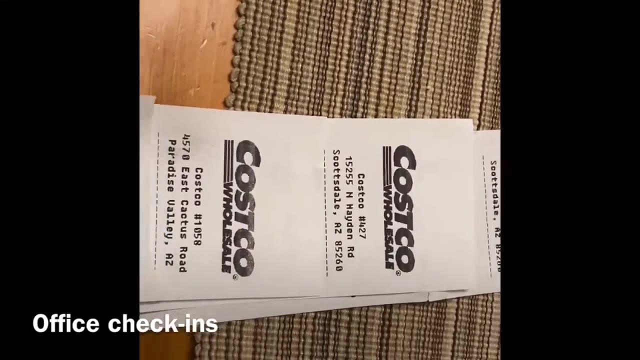 They're having a spinal ablation today. They didn't know they had a device, So we're a page and we get there as soon as possible. So far I've driven probably about 150 miles in the past two days, Rocking that empty gas tank. 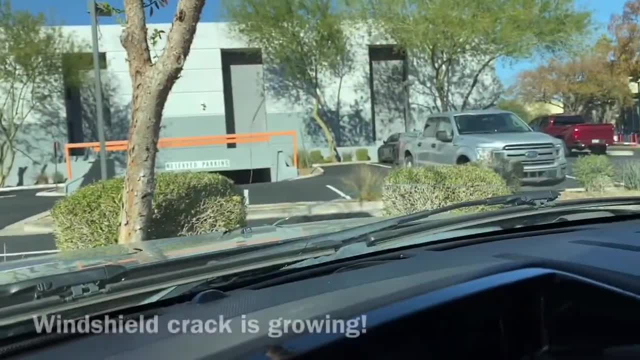 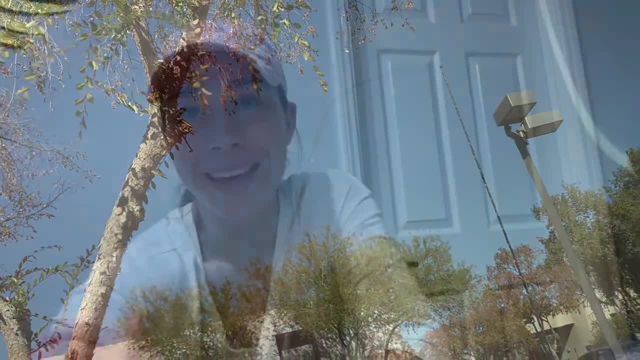 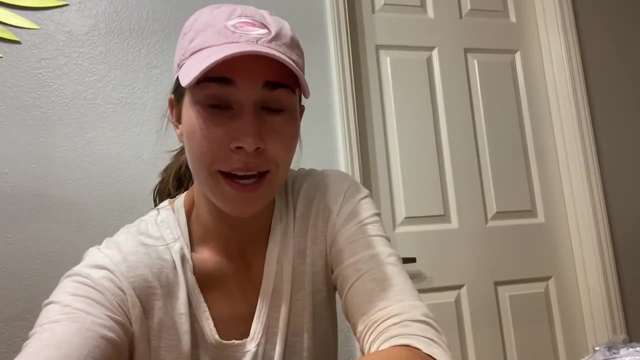 Good thing Costco keeps me fueled up. I just wanted to hop on at the end and just be real with everyone. I lost track of the weeks before New Year's Eve and after New Year's Eve We had a lot of people out with COVID symptoms. 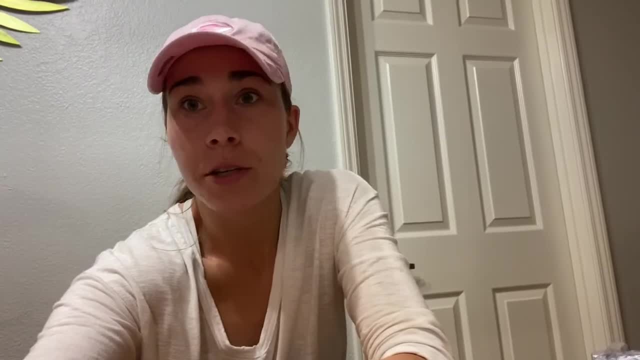 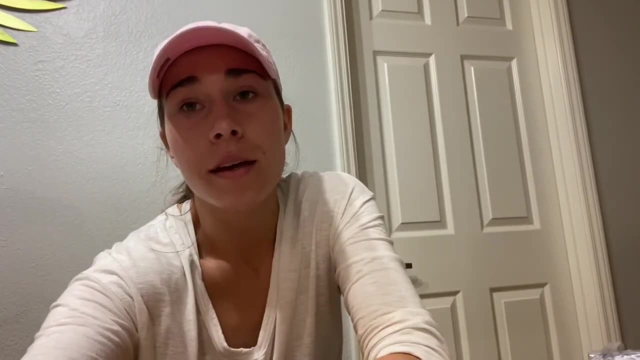 And if you test positive, or someone in your house tests positive, you're just out two weeks and there's nothing around it. So we've been borrowing reps from other areas, For example San Jose, San Diego, anywhere within our West Coast region. 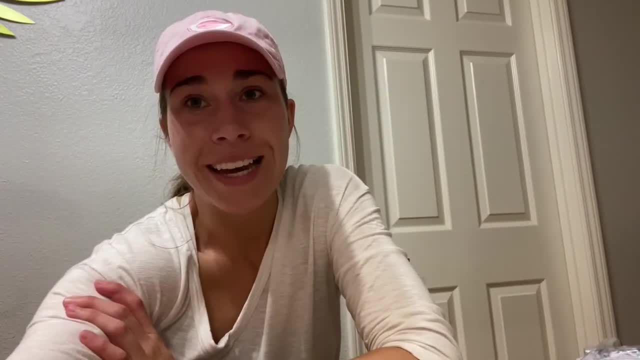 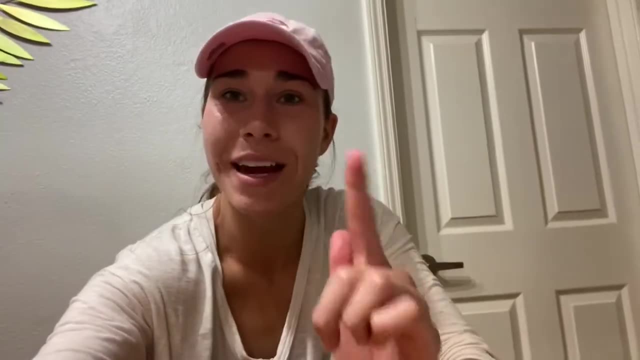 Just so we have enough bodies to get things covered. My days are very full. I honestly really feel like the last woman standing because I haven't had any symptoms. I felt great. I've been careful. I try to get as much sleep as possible. 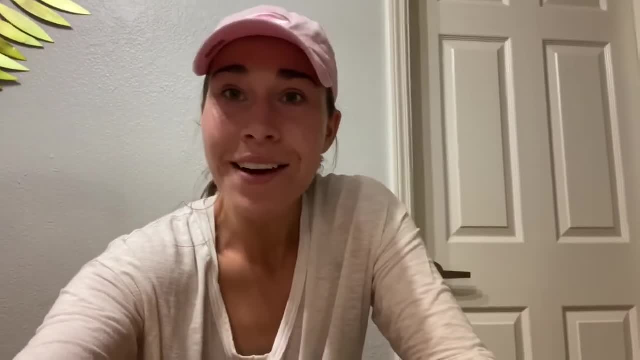 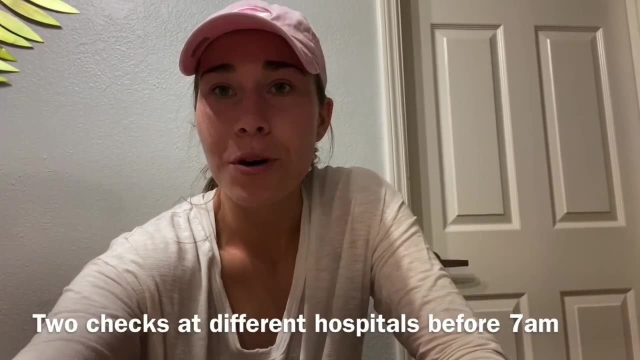 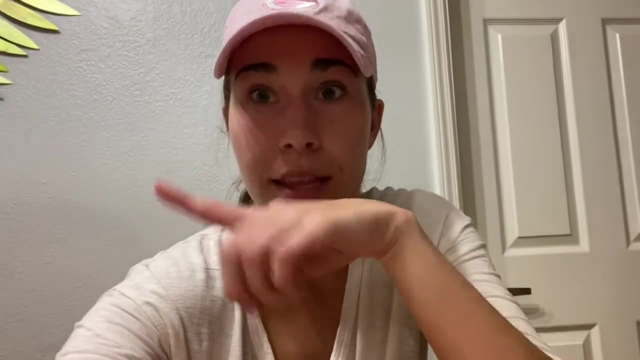 I think that helps And yeah, we're just riding this wave. I will give an example of my Friday. It was two patient discharge checks at two different hospitals before 7 o'clock, Arriving at the third hospital in the morning for a 7.30 case. 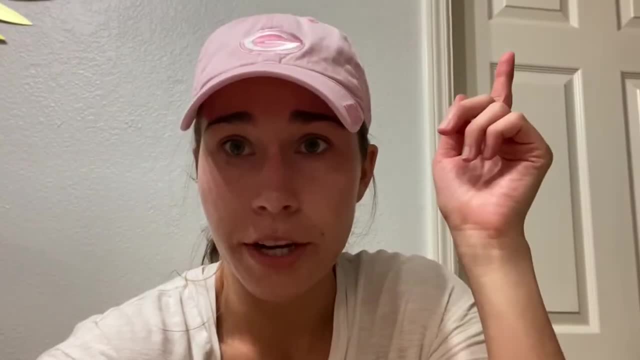 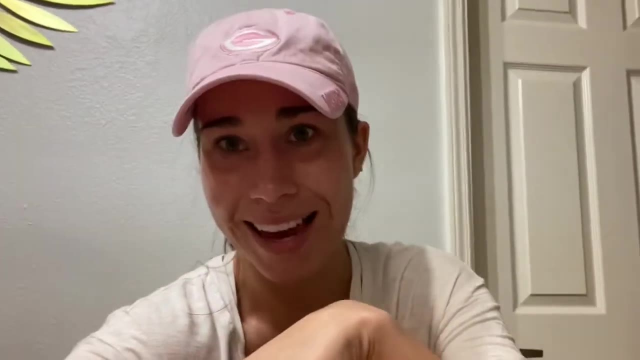 Doing that case: Going to the hospital, Going to the floor to check a patient, Going around the corner to do two MRIs at a different hospital. Coming back to check on timing for my next case- Successful case. However, it took a little longer. 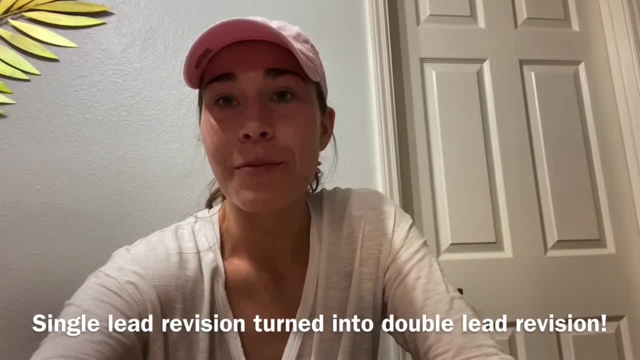 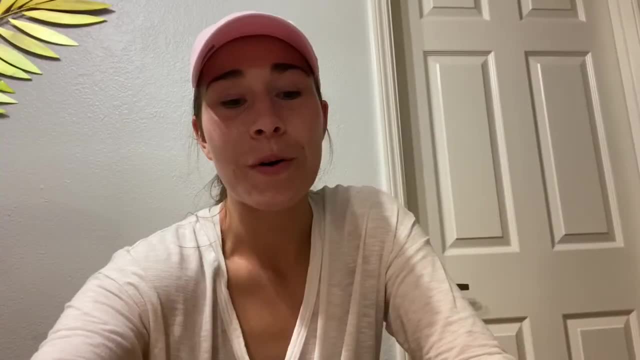 It was a lead revision And while we were after we fixed the first lead and we were stitching up the pocket, Guess what, The second lead pulled back somehow. So we had to go back in and fix that one. We had already sewn the pocket. 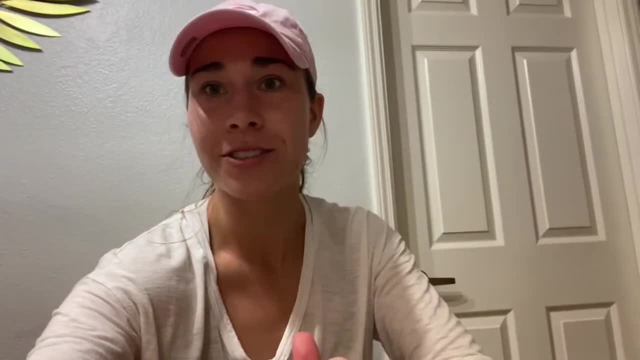 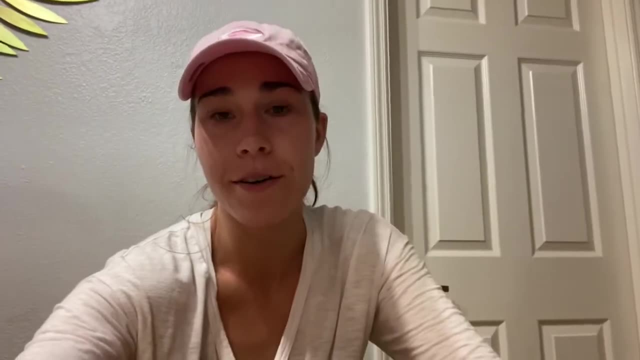 Like patient, was ready to be off the table. My numbers change And I have to be the one that raises my hand and say, Hey doc, Hey doc, My numbers look different, Let's check it out. And then we floro. 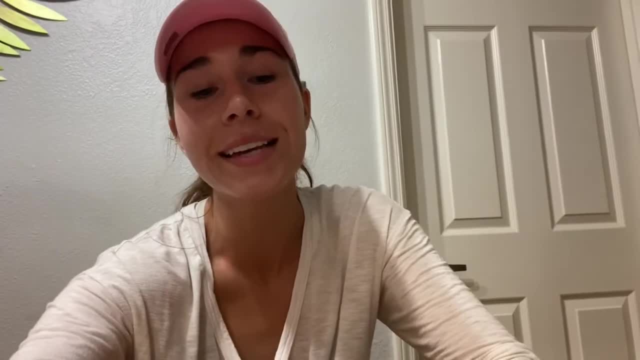 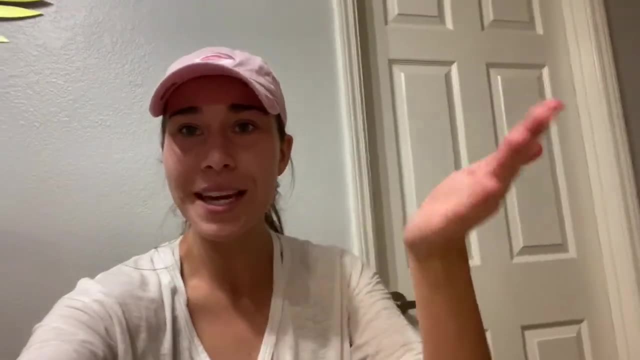 Lead fell back. A case that should have taken about 45 minutes went south and took close to three hours, But that's the nature of the beast. I had another case, but the call team tagged me out, which I'm very thankful.